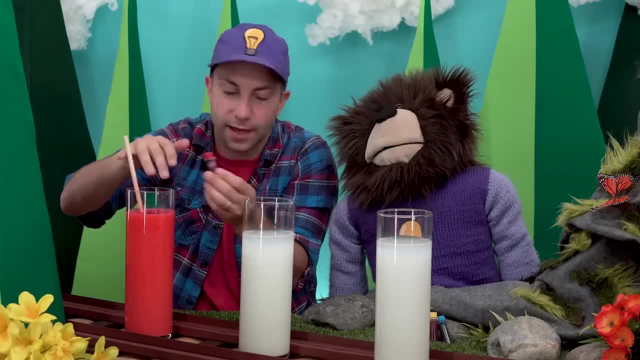 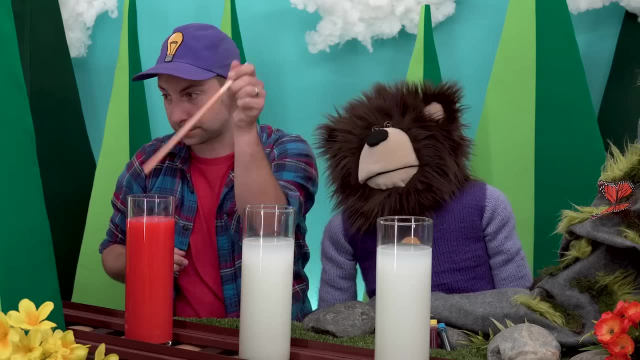 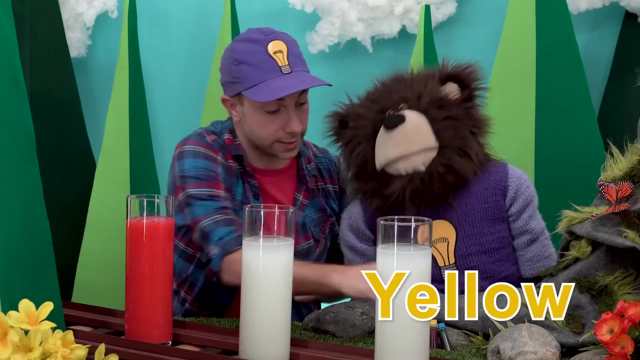 Boop boop, boop, boop boop. Close that up And stir again. There we go. It's nice and bright, Wow. Okay, Meta, let's add the yellow dye to the second container, Alright. 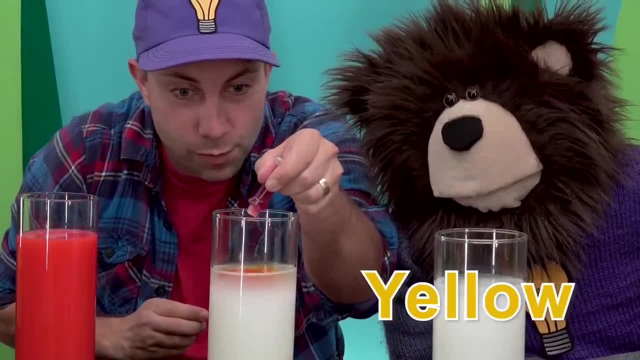 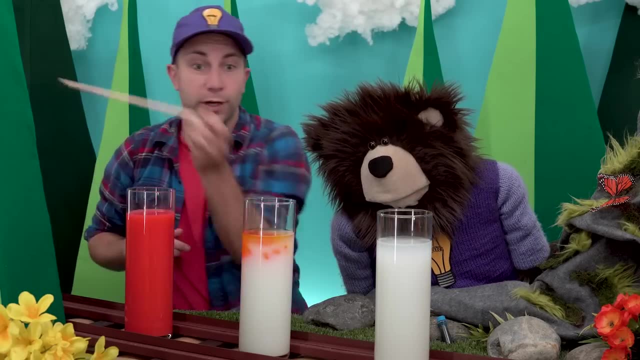 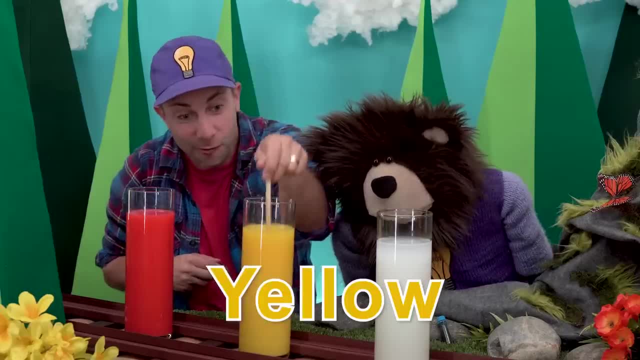 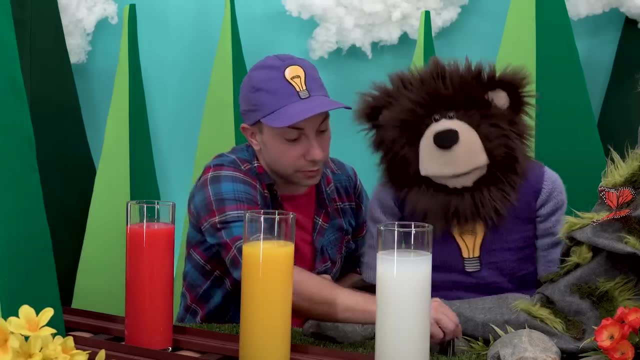 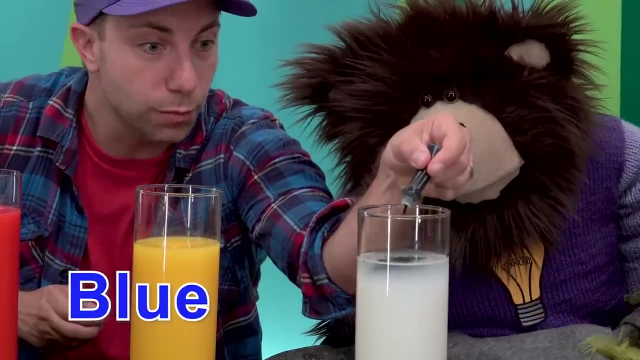 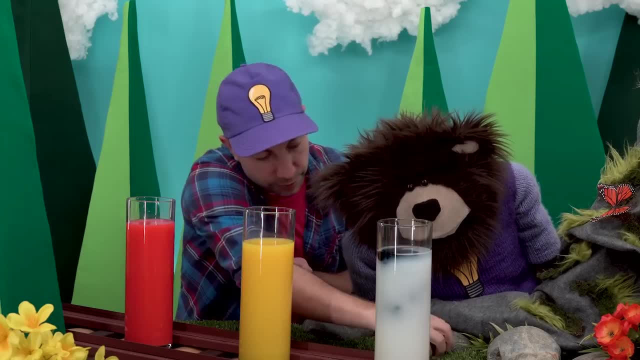 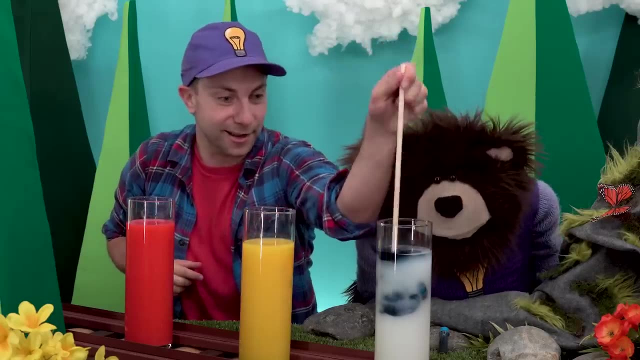 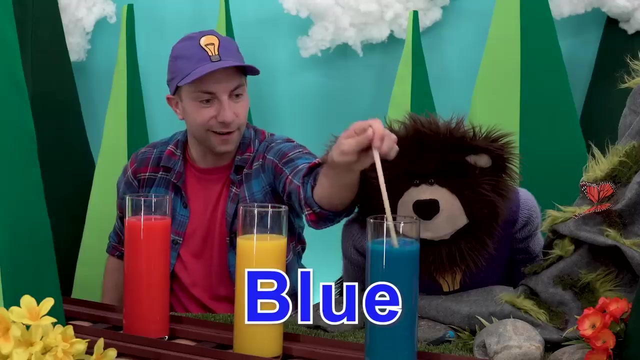 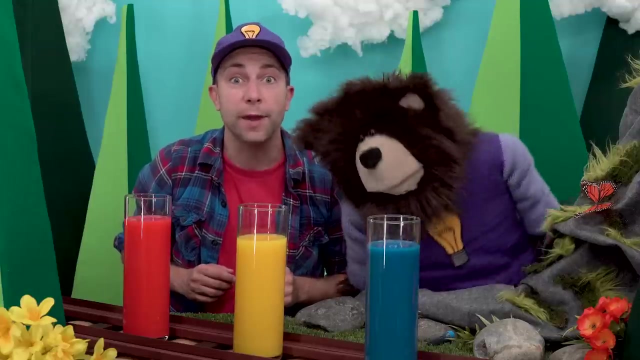 Boop. Okay, Now we will take the wooden stick and mix it up. Are you ready, Meta? Yes, Okay, Here we go. Whoa, Look at that, Meta, It's turning blue. These three colors are called primary colors: Red, yellow, 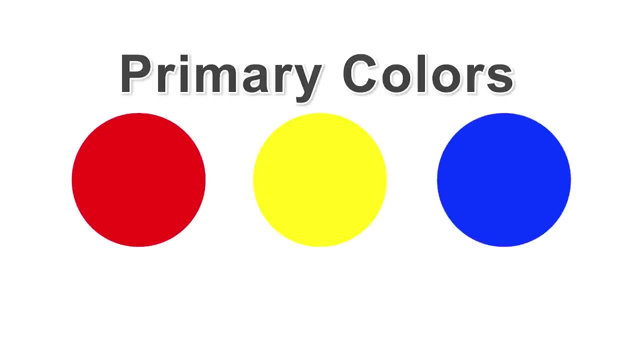 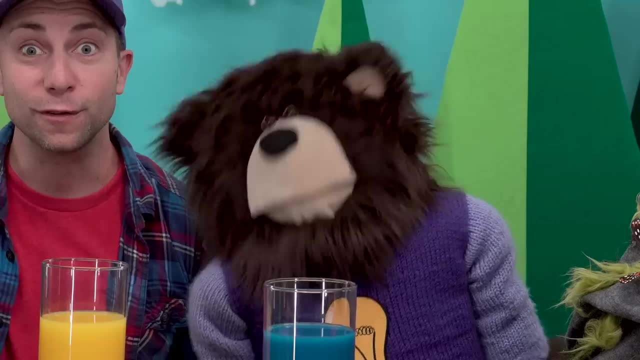 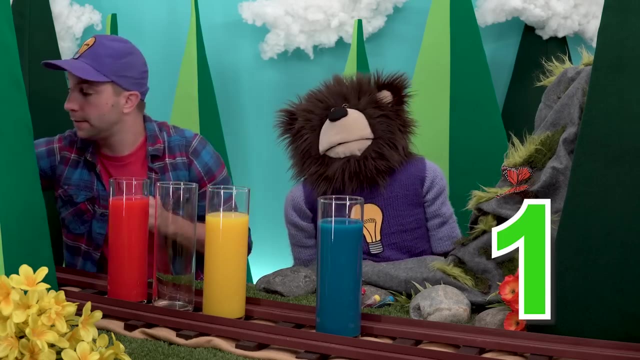 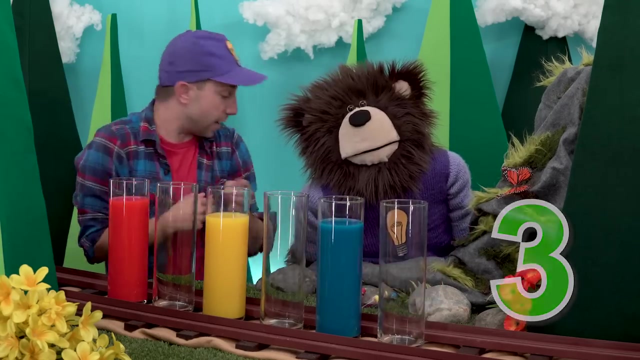 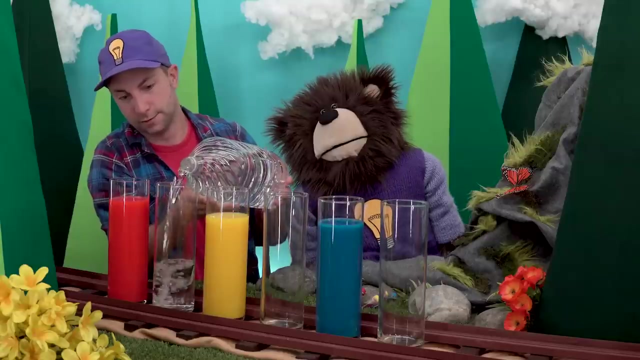 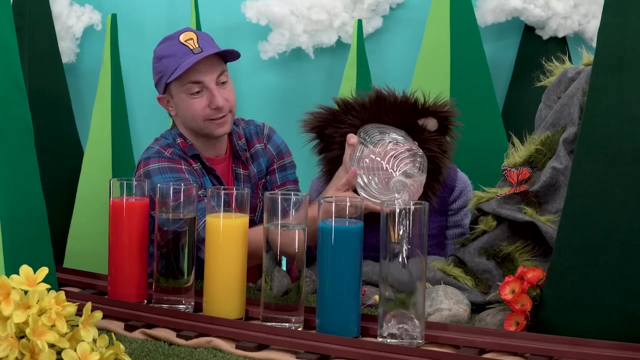 and blue are called primary colors. Okay, Are you ready to mix some of these primary colors to make new colors? Yes, Okay, Meta, I have three more glass containers: One, two and three. Again, we will add our water. Alright, Now we will add our splash of milk. 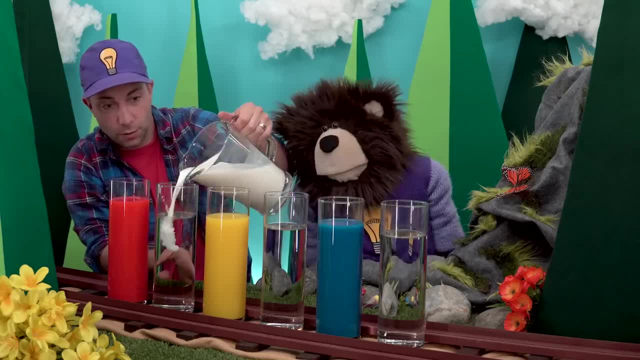 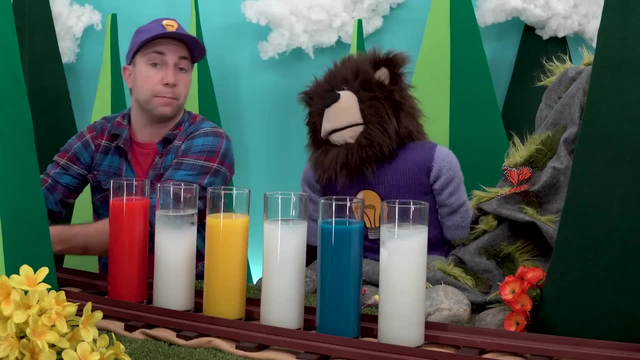 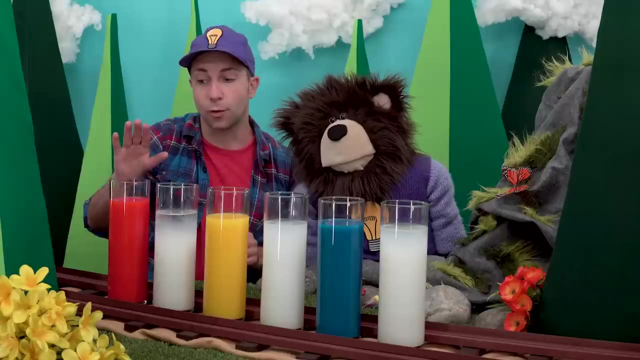 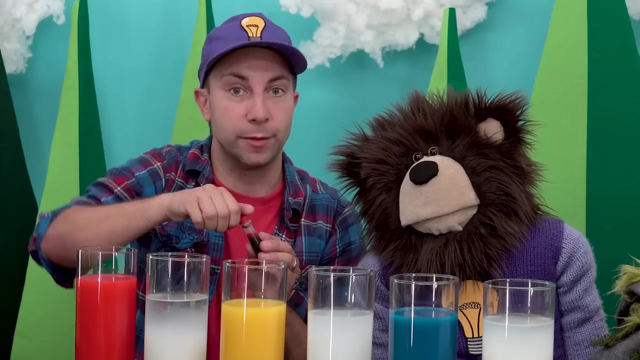 to each one of these containers. Again, the milk helps our colors appear nice and bright. Now, Meta, what do you think will happen if we mix red with yellow? Let's find out, Alright. So first we will take our red dye and add two drops. One, two. 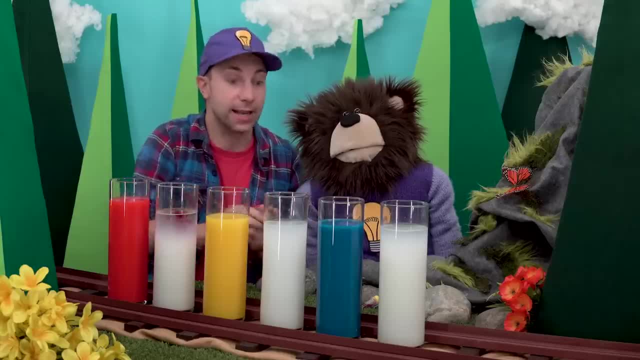 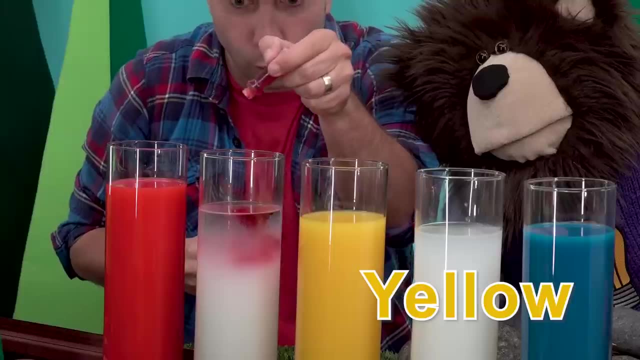 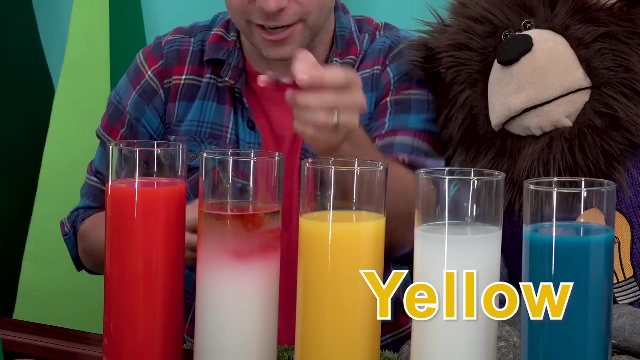 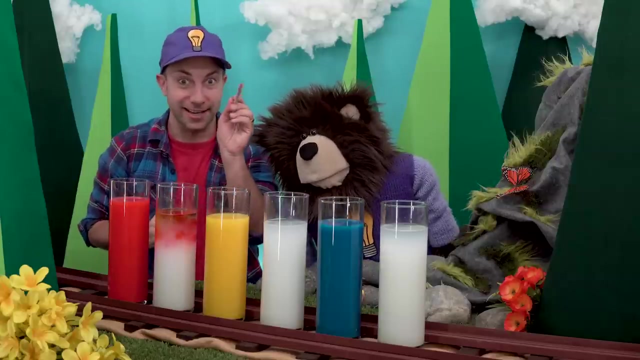 Alright. Next we will take our yellow dye and add five to six drops: One, two, three, four, five, six, One more Seven. Okay, Now we will take the wooden stick and mix it up. Are you ready? Here we go. 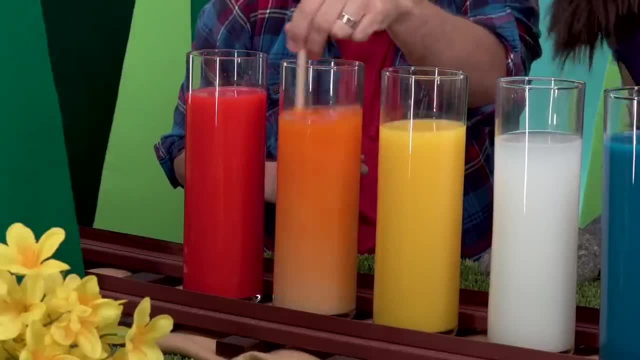 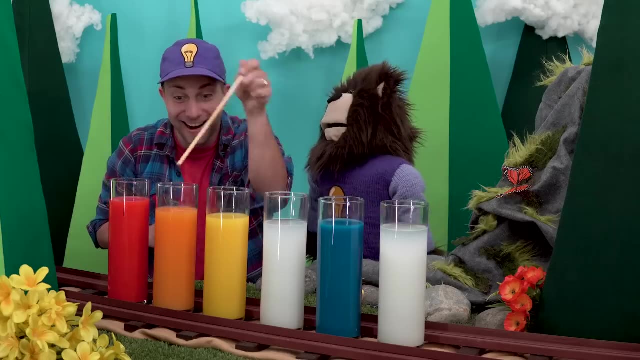 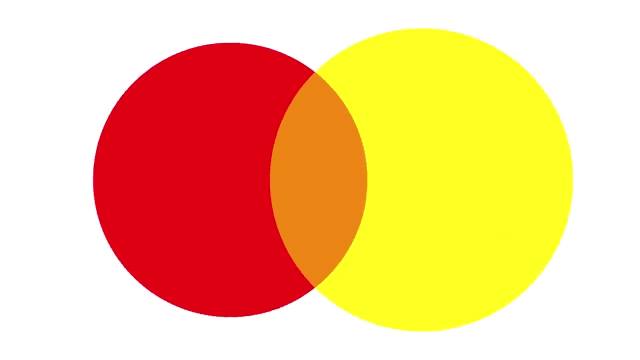 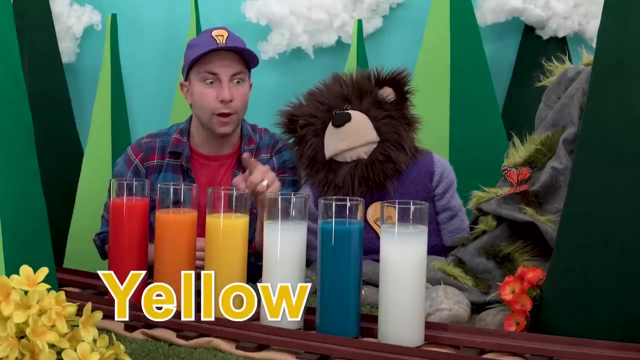 Whoa Meta, Look at that. Mixing red with yellow makes orange. Wow, That is really neat. Red mixed with yellow makes orange. Are you ready to make another color? Alright? What do you think will happen if we mix yellow with blue? Let's. 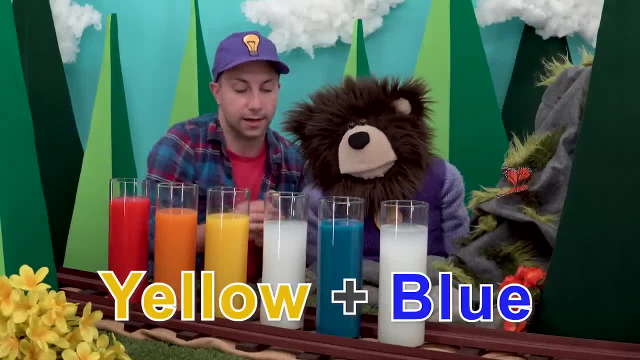 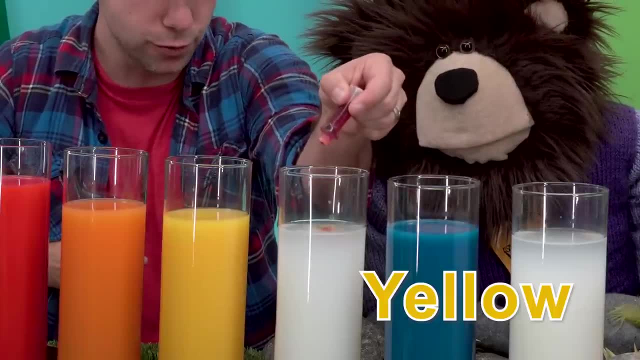 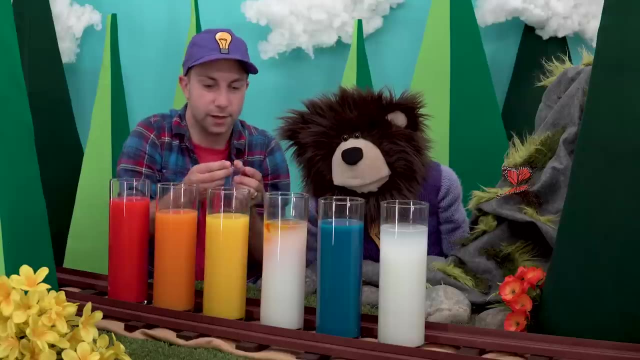 find out. First we will take the yellow dye and add about five to six drops: One, two, three, four, five, six. Okay, Let's add another drop, Meta. Alright. Now we will take our blue dye and add two drops. 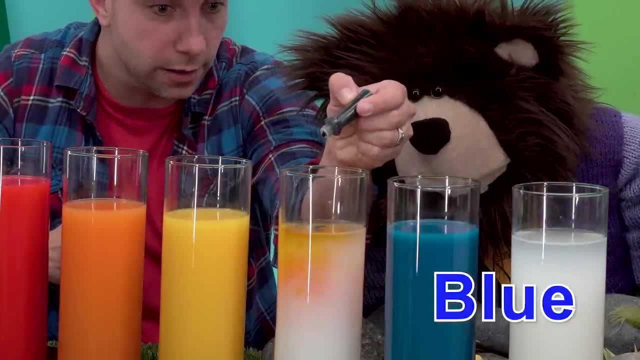 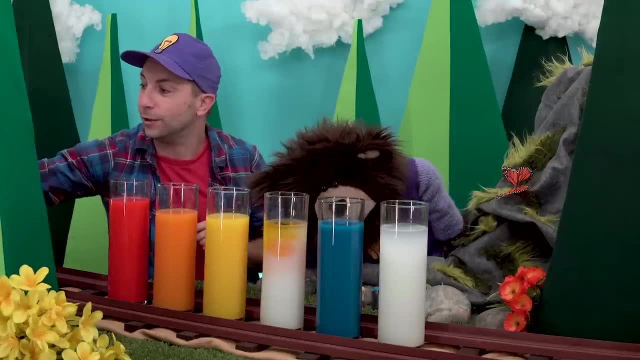 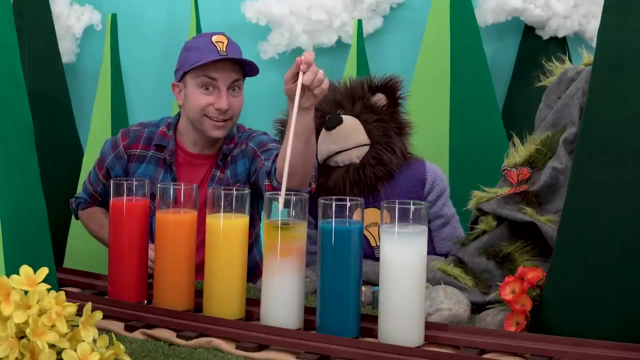 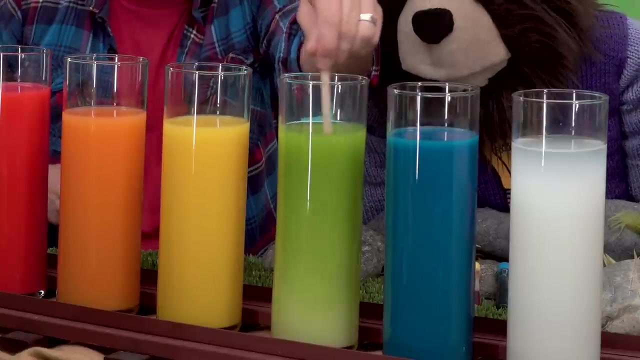 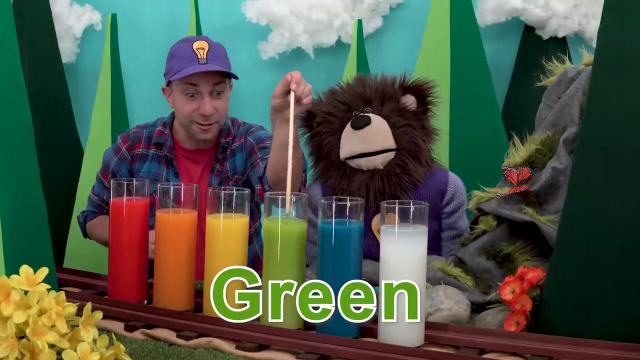 One, Two. Okay, We will take a wooden stick and mix it up. Are you ready to see what color we are making? Yes, Okay, Whoa, Meta, Mixing yellow and blue makes green. Wow, Look at that. Yellow mixed with blue makes green. 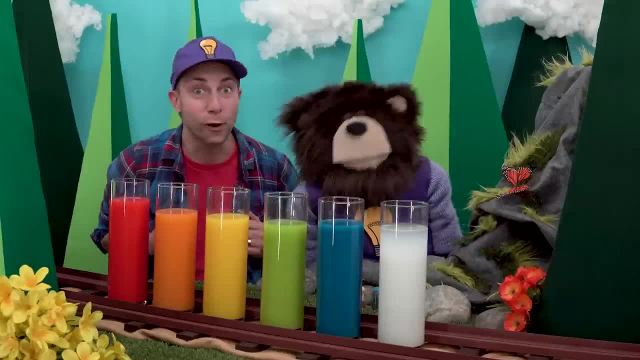 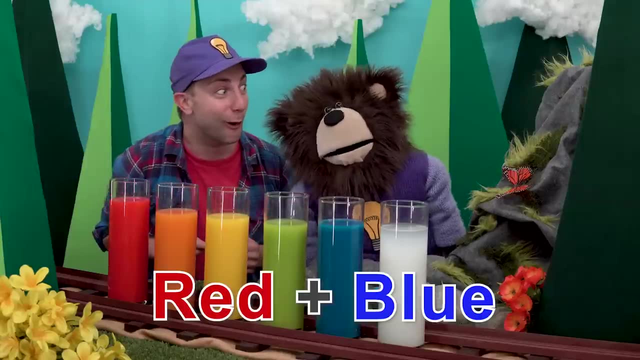 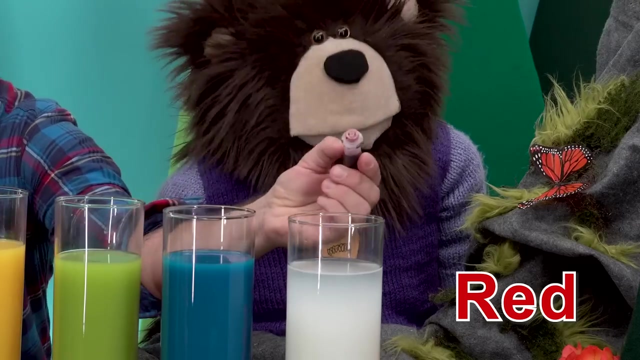 Let's make one more color. What do you think will happen if we mix red and blue? Oh Okay, So let's take our red dye and we will add about four to five drops: One, two, three, four, five. 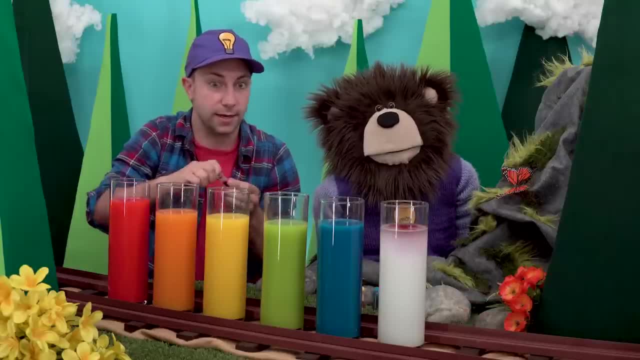 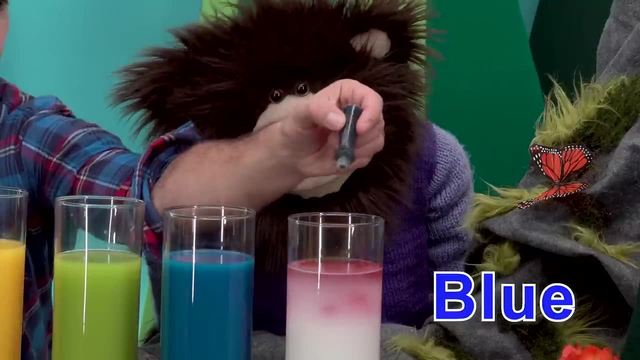 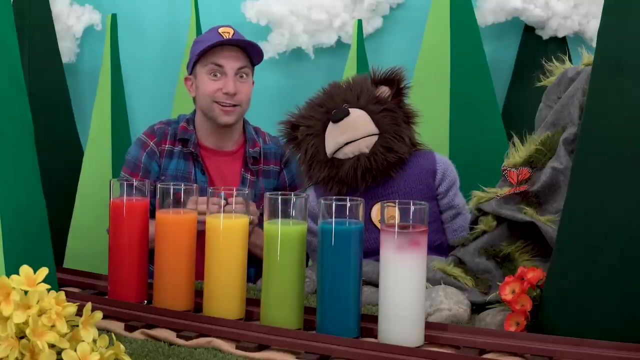 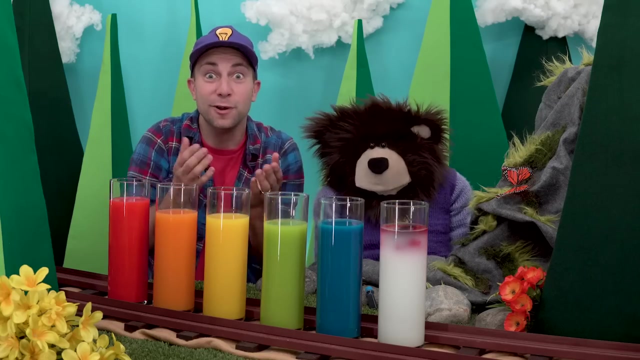 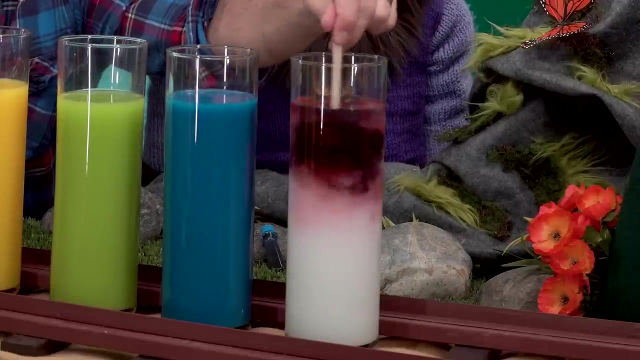 Alright, One more. Then we will take our blue dye and add two drops. One, Two. What color do you think we are making, Meta? Do you know? Let's find out. Okay, Take the wooden stick and mix it up. 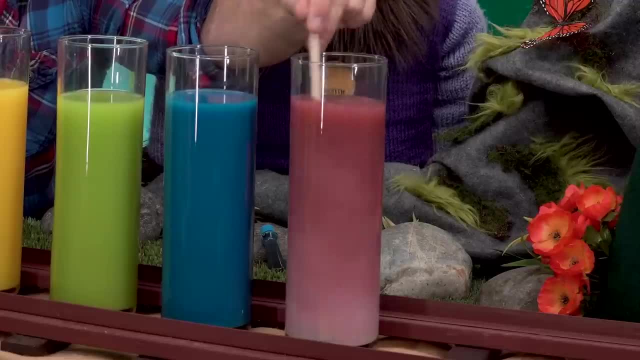 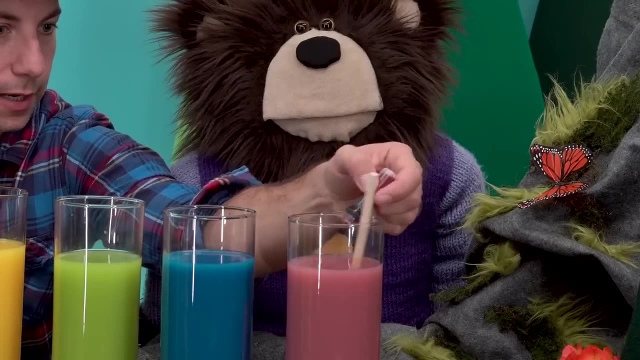 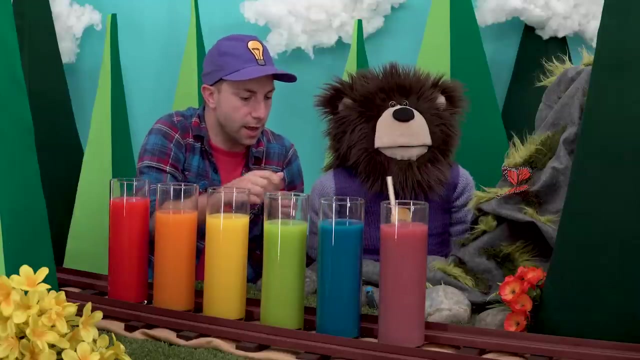 Whoa, Look at that Meta. Let's add a few more drops of red to really make it nice and bright. Okay, Oh, We are going to need to add a few more drops of blue. Boop, boop, boop, Let's see. 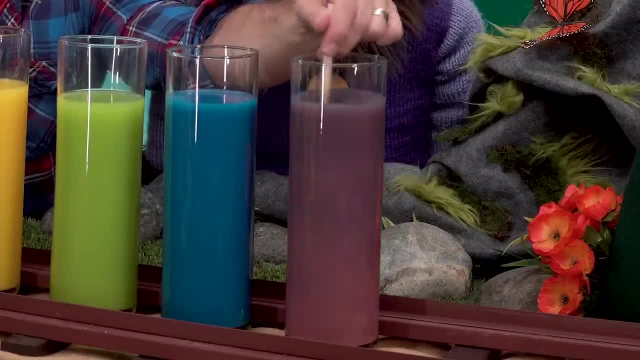 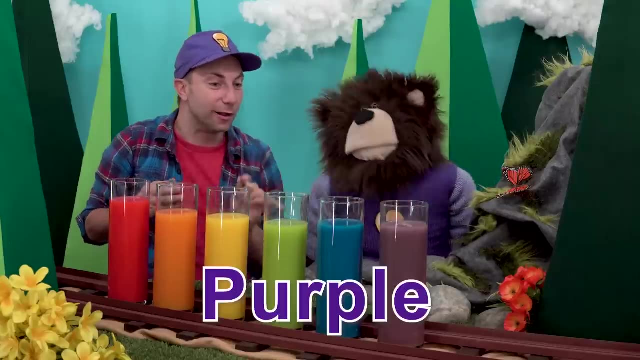 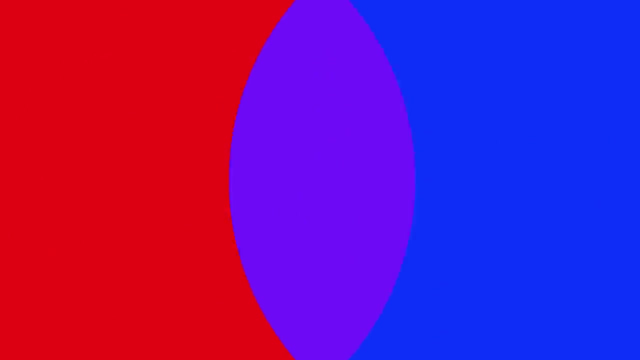 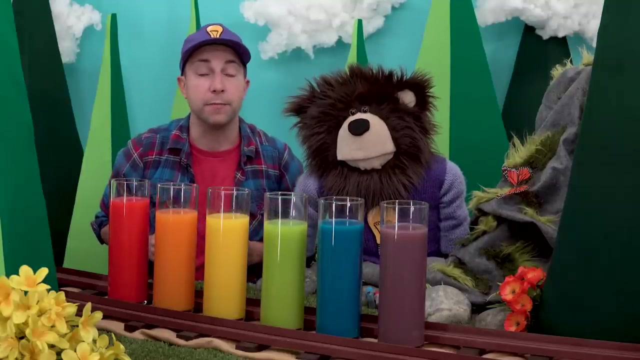 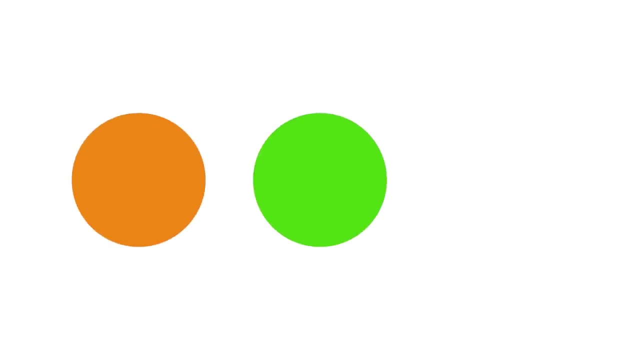 Oh, There it is, Meta. Look at that. That is the color purple. Wow, Red mixed with blue makes purple. These three new colors- orange, green and purple- were made by mixing primary colors. They are called secondary colors: Orange, green and 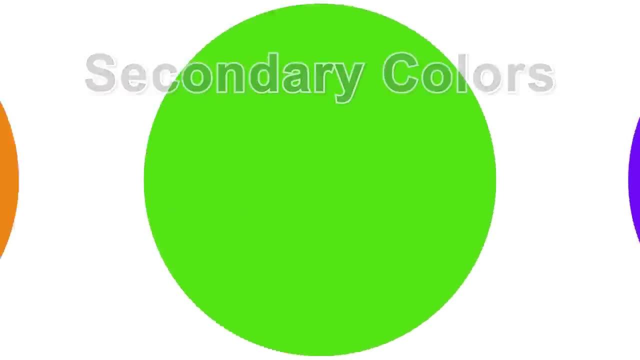 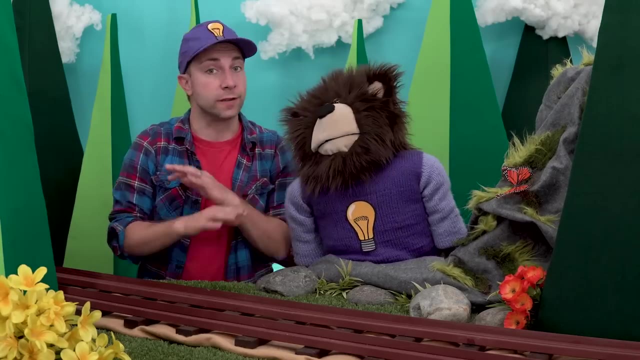 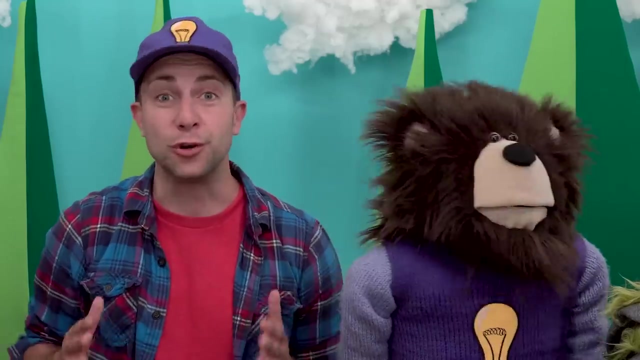 purple are called secondary colors. Do you know what time it is? It's time to dance. This is where we stop what we are doing. stand up and dance. You can do whatever dance move you feel like doing. Do you hear that? It's the idea train. 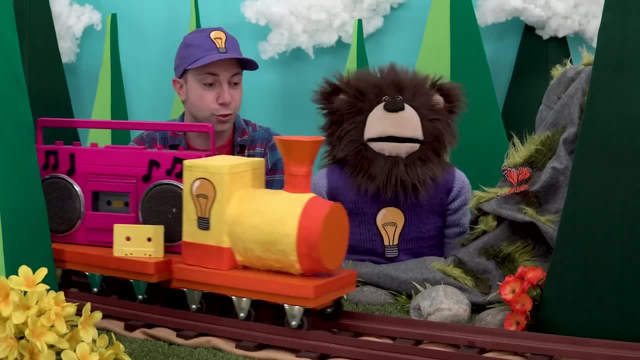 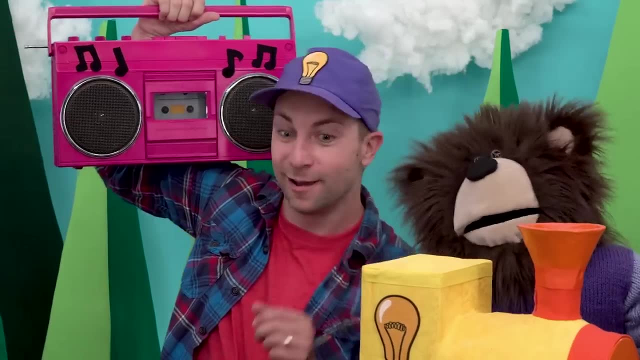 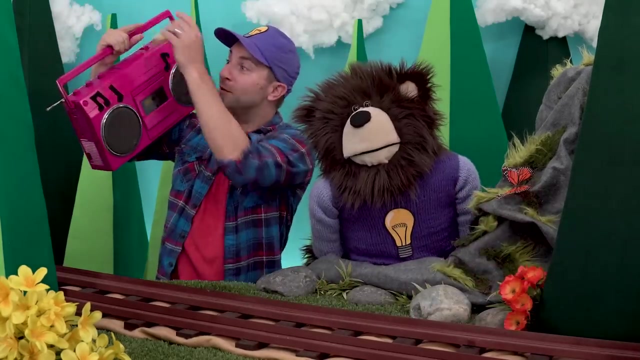 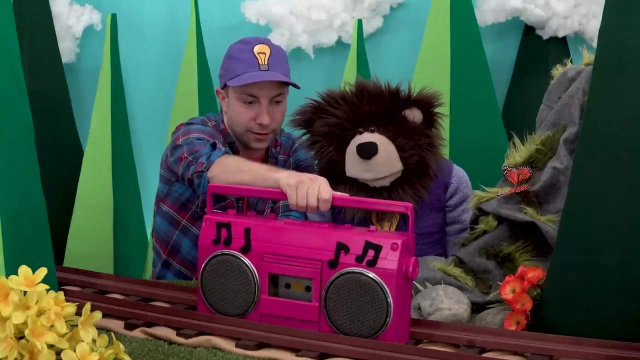 And look, It's Pinky the Boom Box. Hi, Pinky the Boom Box. Alright, Thank you, idea train. Oh, Pinky the Boom Box plays our music. We will put Pinky right here. Then we will take this yellow cassette tape. 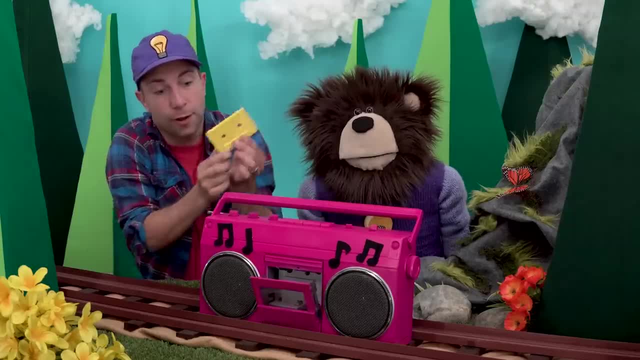 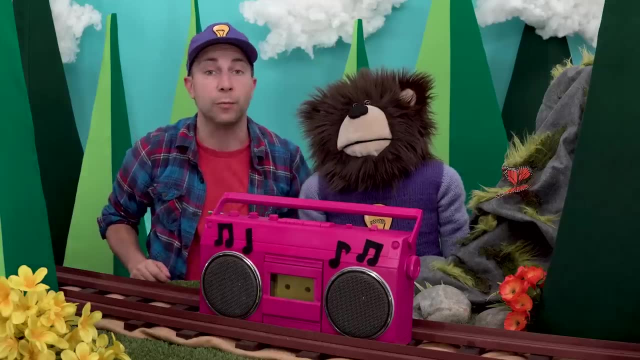 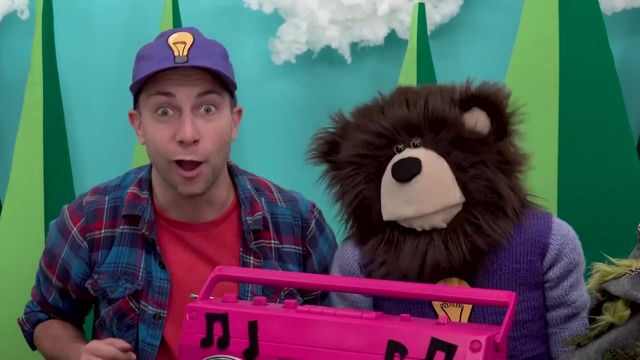 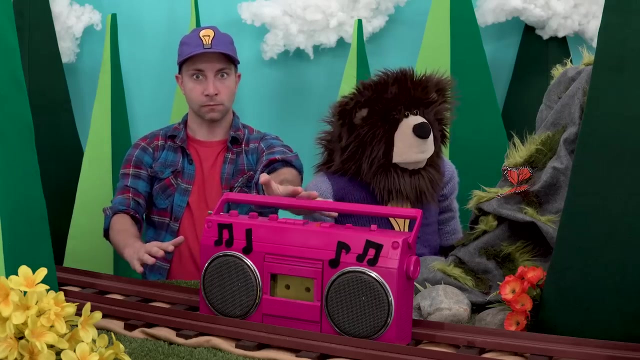 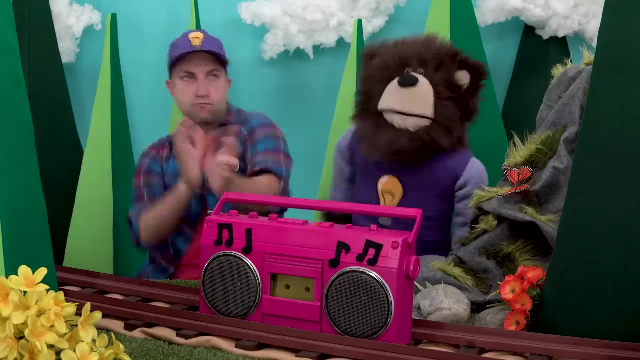 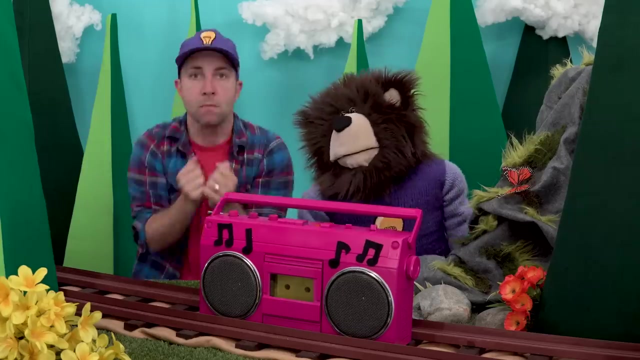 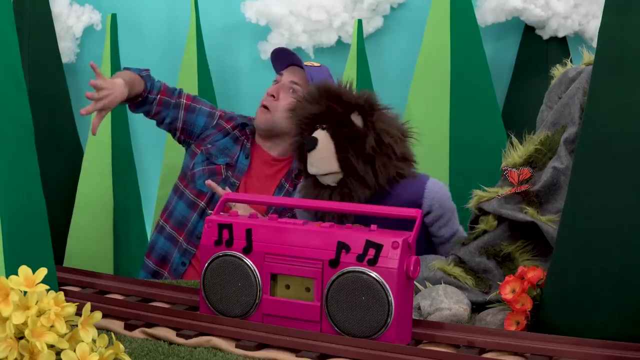 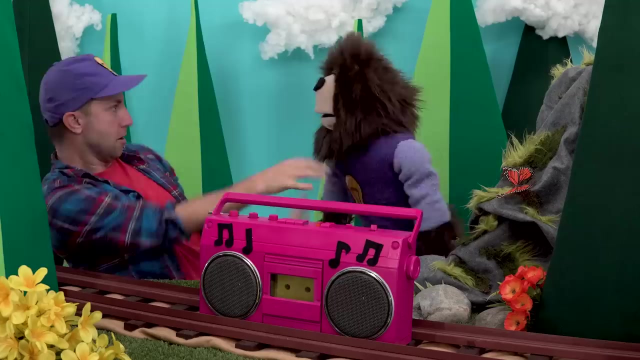 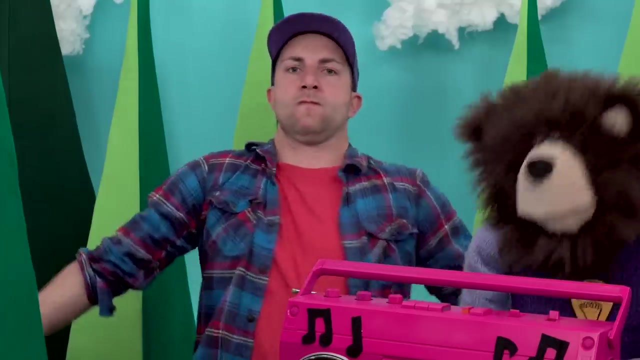 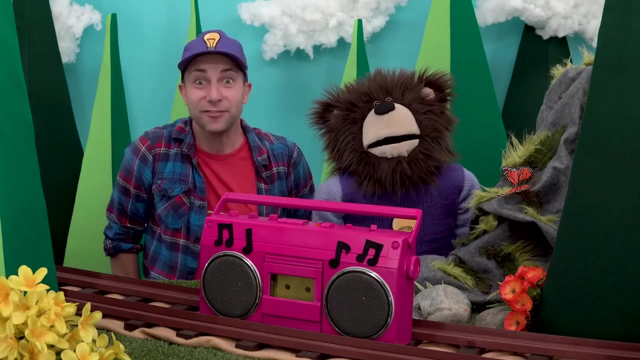 and put it in here, and then we will close it up. then we will push the button with the triangle on it- the play button. are you ready to dance? yes, okay, I'm going to push the play button now. Oh, that was a lot of fun. okay, let's get back to what we were doing before we go. 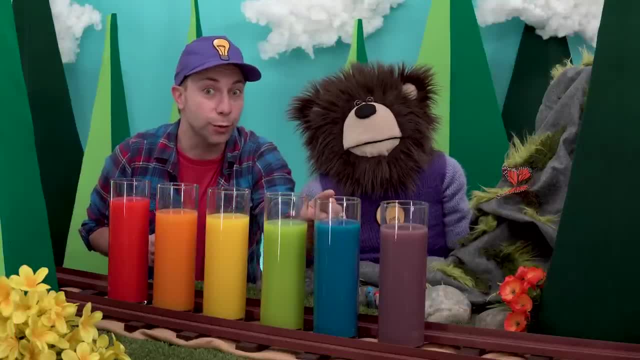 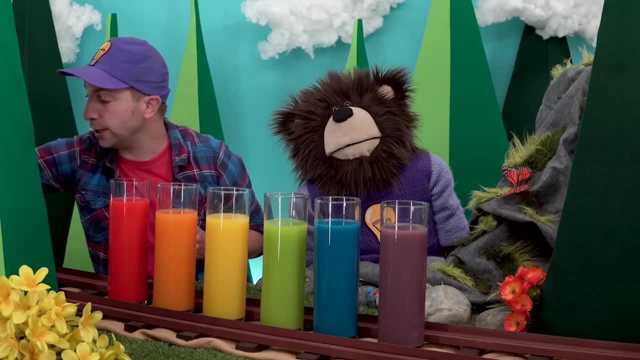 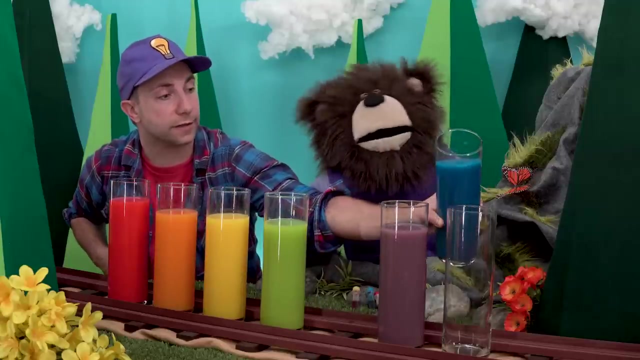 what do you think will happen if we mix the color blue with the color purple? should we find out, Mayta? yes, okay, I have one last glass container. we will pour half of our blue color into this container. are you ready, Mayta? mm-hmm, here we go. 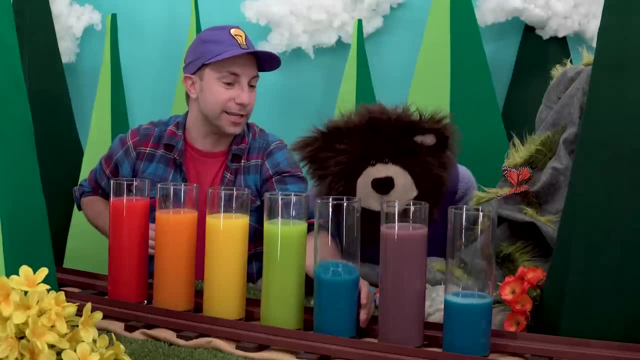 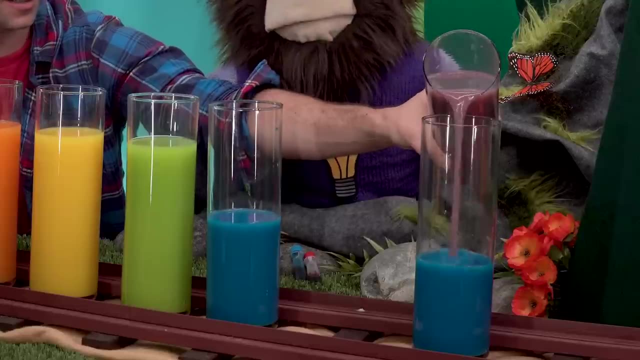 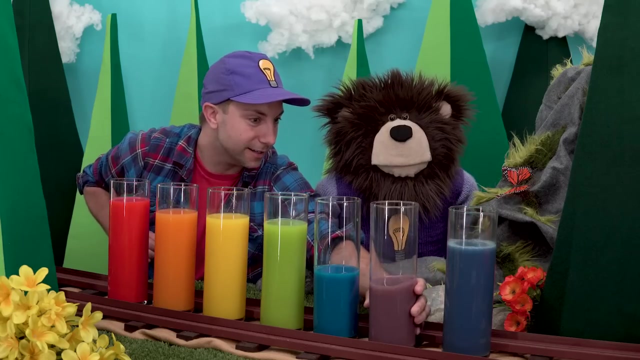 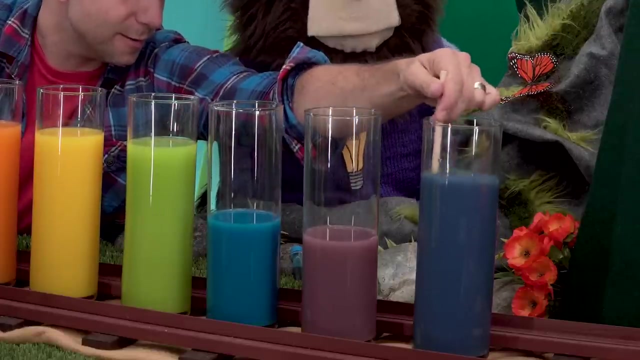 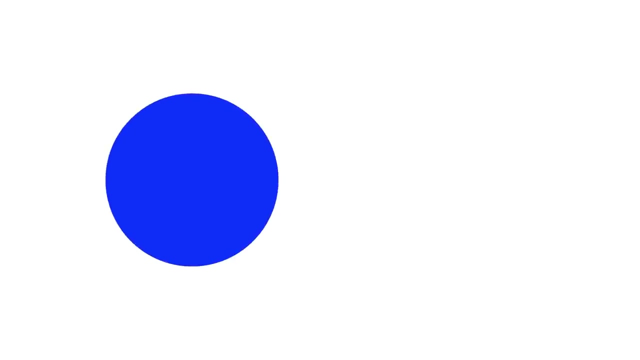 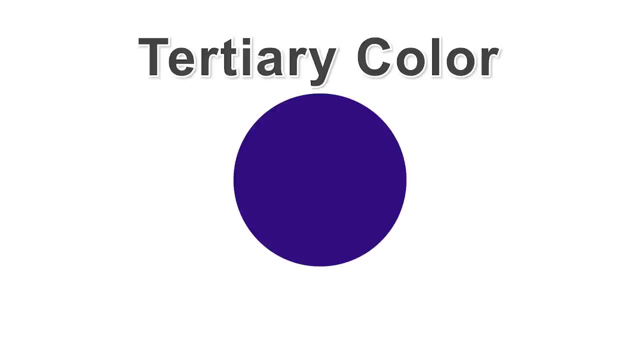 whoa. now we will take our purple and pour half of the purple into the same container. okay, now let's take a wooden stick and really mix it up. wow, That is the color. indigo. Blue mixed with purple makes indigo. Indigo is called a tertiary color. 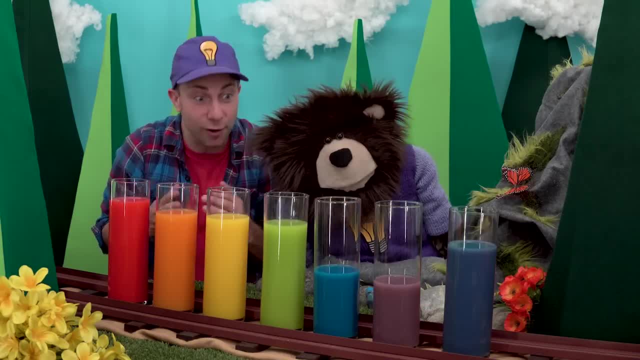 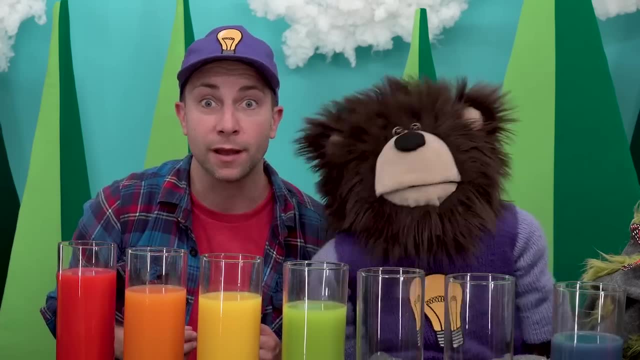 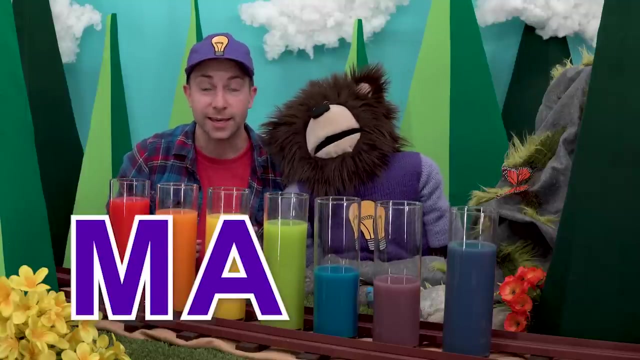 Wow, that was a lot of fun making all these colors. If you want to watch more Meta videos, search Meta's name. Do you know how to spell Meta's name? Let's do it together: M-A-Y-T-A- Meta.